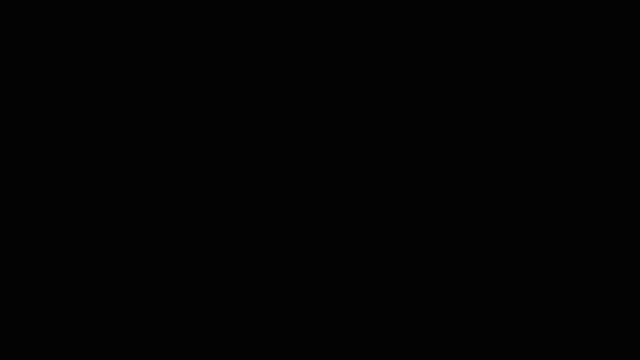 In this video we're going to talk about the difference between a nucleotide and a nucleoside, And then we're going to talk about the difference between purines and pyrimidines. So what is the difference between these two? What is the difference between a nucleoside and a nucleotide? 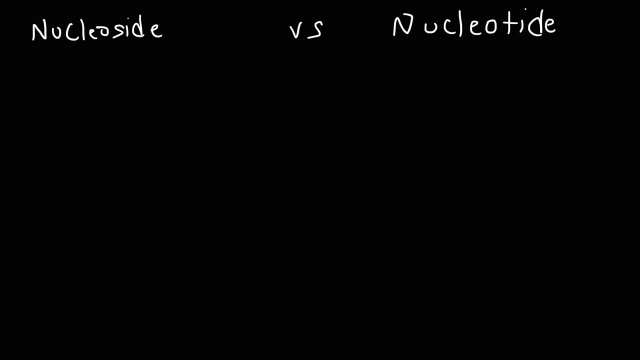 What would you say? A nucleoside has two components to it: It contains a 5-carbon ribosugar and it contains a nitrogenous base. So that is a nucleoside. A nucleotide has three units: It has the 5-carbon ribosugar and it has the nitrogenous base. 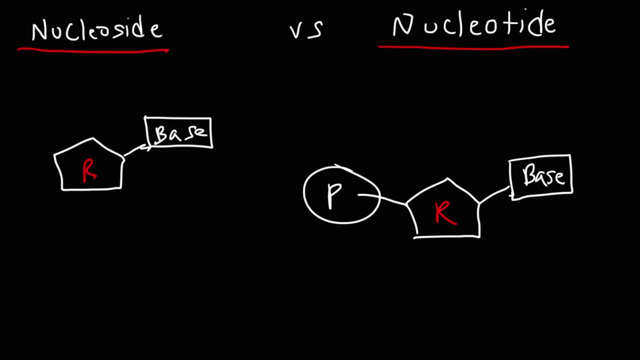 In addition to that, it contains a phosphate group, So that is a nucleotide and this is a nucleoside. Now there are five nitrogenous bases that you need to be familiar with: A, G, T, C and U. 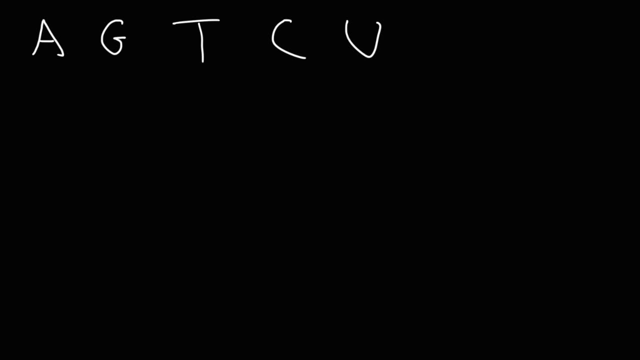 A stands for adenine, G is guanine, T is thymine, C is cytosine and U is uracil. The first two, adenine and guanine, are known as purines. Purines are nitrogenous bases that contain two rings. 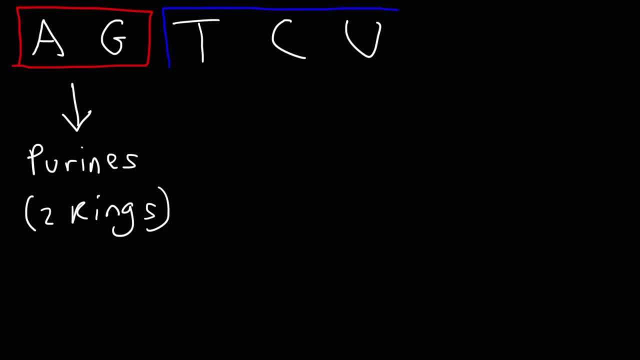 The other three, thymine, cytosine and uracil. these are known as pyrimidines, And the reason for that is that they contain only one ring. So pyrimidines are nitrogenous bases with one ring. 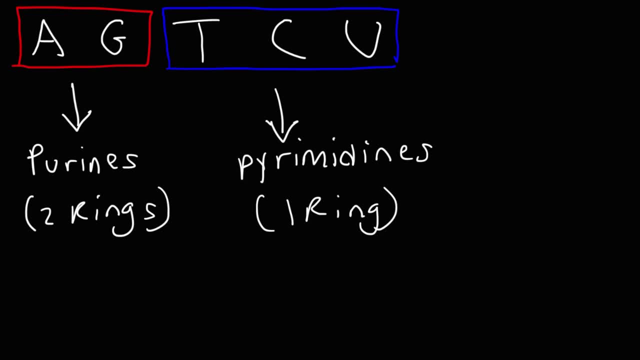 Purines are nitrogenous bases with two rings. Now it's important to know that DNA deoxyribonucleic acid contains the nitrogenous bases A, G, T, C. RNA ribonucleic acid contains the bases A- G. 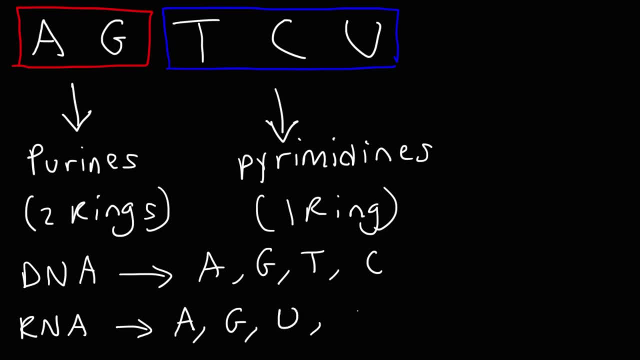 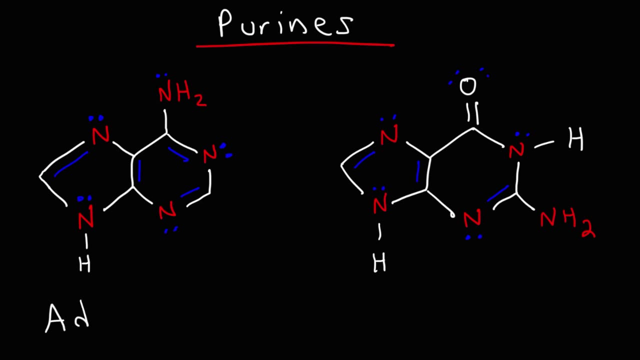 Now, instead of thymine, RNA has uracil. So make sure you understand that DNA contains thymine, but RNA contains uracil. So here we have two purines. On the left we have adenine. 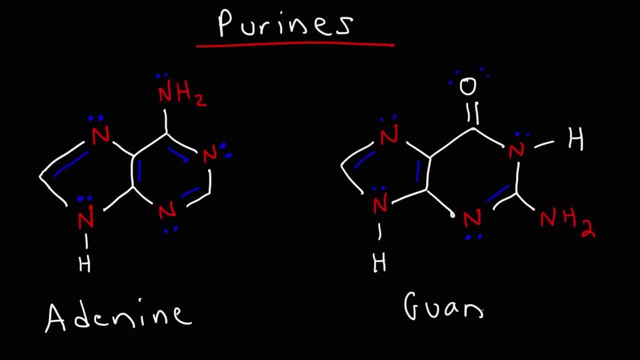 and on the right. this is guanine. One key difference between the two is that guanine has a carbonyl group, whereas adenine does not. Adenine does have this aromatic ring. It looks like a benzene ring, but it's a heterocyclic aromatic ring. 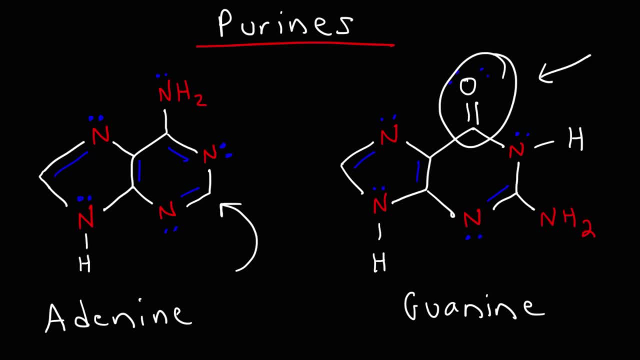 due to the nitrogen atoms. Whenever you see a six-membered ring with alternating double bonds, such a ring is very stable. So you can see that this is a heterocyclic aromatic ring due to the nitrogen atoms. Whenever you see a six-membered ring with alternating double bonds, such a ring is very stable. 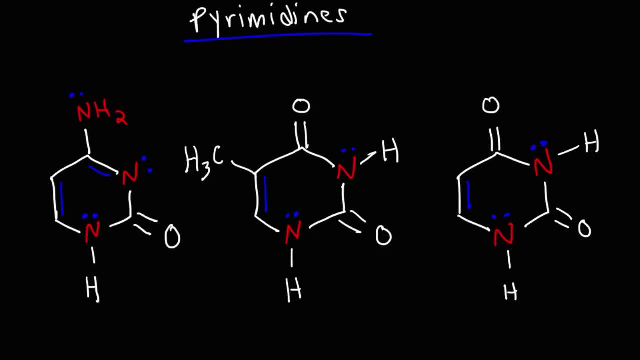 Due to aromaticity. So here are the structures of the three nitrogenous bases that are pyrimidines. They contain one ring. On the left we have cytosine, In the middle thymine And on the right uracil. 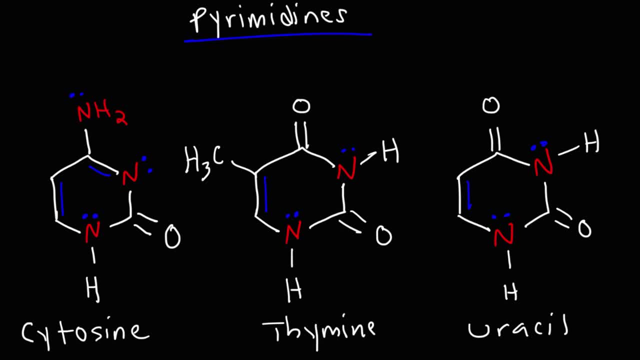 Notice that thymine and uracil look very similar. The only difference is that thymine has a methyl group, whereas uracil has a methyl group, Whereas uracil does not. Now, both thymine and uracil contain two carbonyl groups. 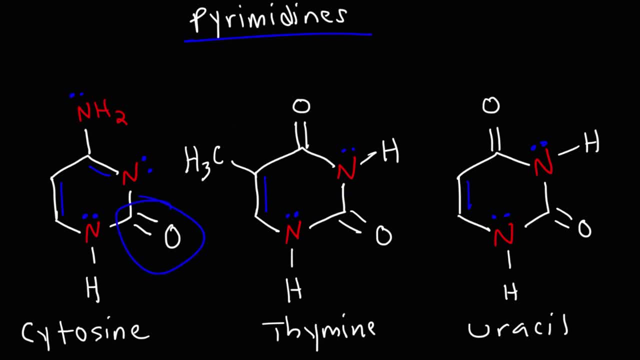 whereas cytosine only contains one. So that's how you can tell them apart. Cytosine has one carbonyl group, thymine has the methyl group, and uracil just has two carbonyl groups and two nitrogen atoms. 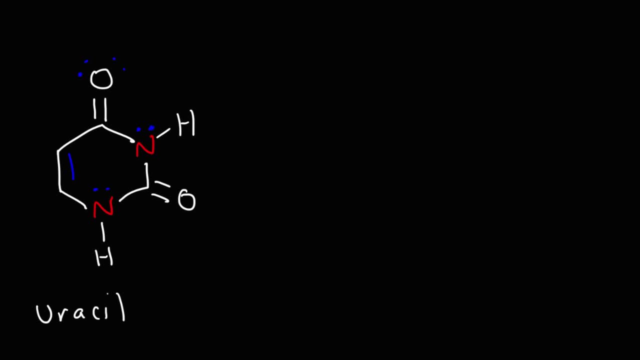 Now the pyrimidine molecules are quite stable because if we draw the resonance structure, you could see that they could form an aromatic ring. Let's take a lone pair from nitrogen and let's use it to form a pi bond, And let's break the pi bond of the carbonyl group. 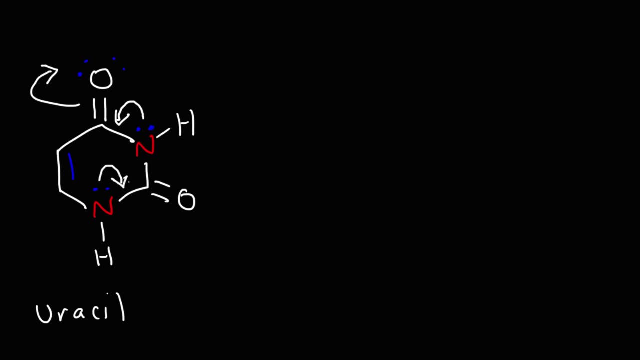 Now let's do the same thing with the lone pair on the other nitrogen atom. This oxygen also has two lone pairs, but once we break the pi bond it's going to have three lone pairs, And so we're going to get a resonance structure.